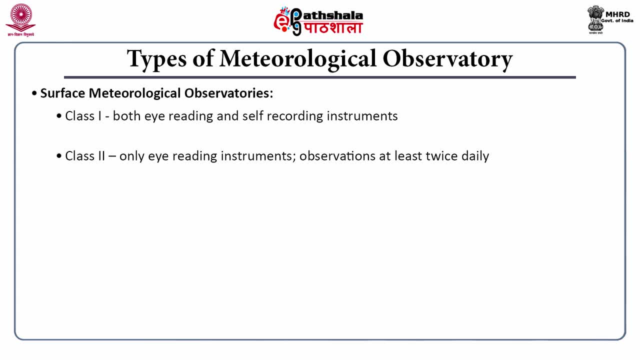 instruments are there. In class 2,, only eye reading instruments are there and observations are taken at least twice daily. In class 3,, only eye reading instruments are there and observations are taken once daily. In case of class 4,, 5 and 6, lesser number of instruments are there. 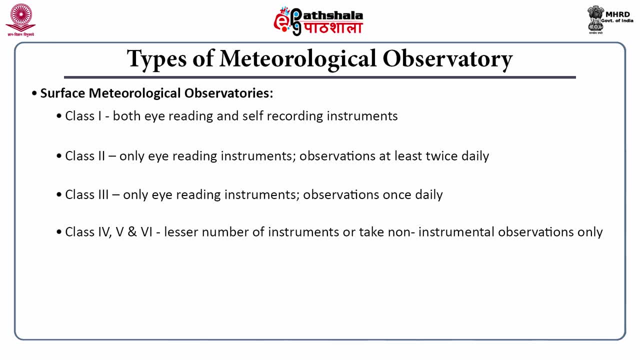 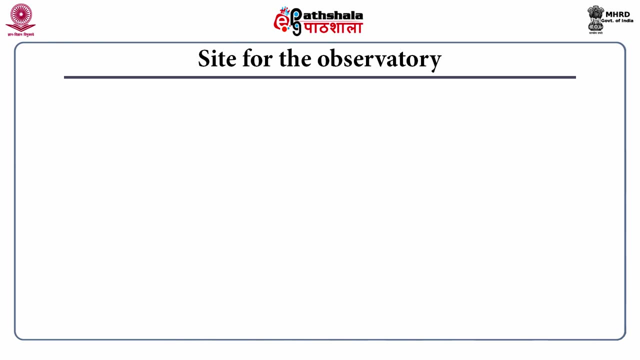 or, in some cases, non-instruments. observations are taken only In case of agronomic observatories. they have been classified into three types. One is principal type, then ordinary and third one is auxiliary type. Now, what should be the ideal site for the observatory? The IMD, which is the nodal agency? 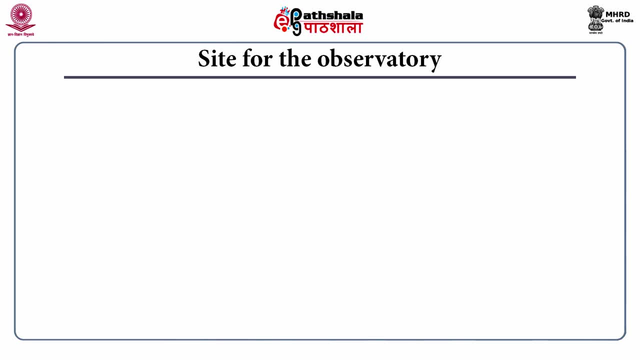 of weather observations and weather services in this country. they have prescribed the standard size, which is 55 meter along north- south direction and 36 meter along the east west direction. A well exposed- it should be a well exposed- bare plot, level plot and 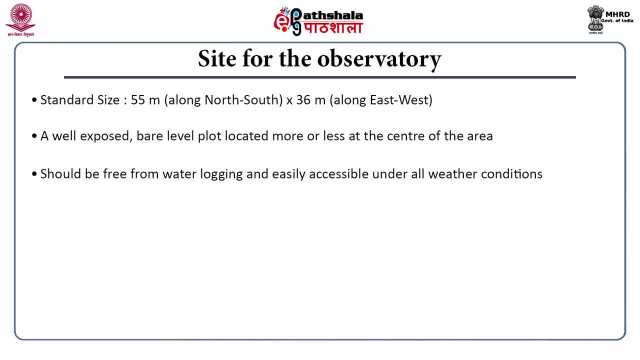 located more or less at the center of the area. It should be free from water logging and should be easily accessible to the public. It should be easily accessible to the public. It should be easily accessible to the public. It should be easily accessible to the public. 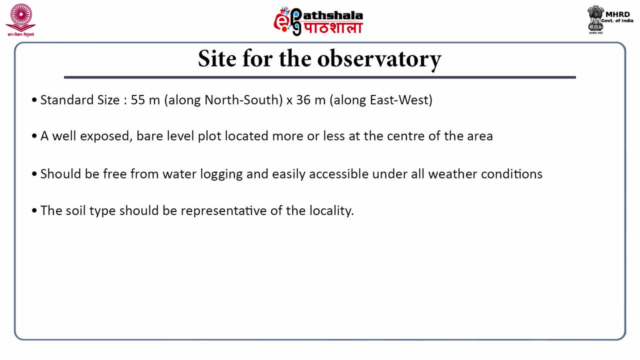 which is really suitable under all weather conditions. The soil type of the observatory should be representative of that locality. It should be a good distance away from the large obstructions like tall trees, buildings, main irrigation or drainage channels, etc. Also, it should be properly fenced with barbed wires for safety of the instruments as well. 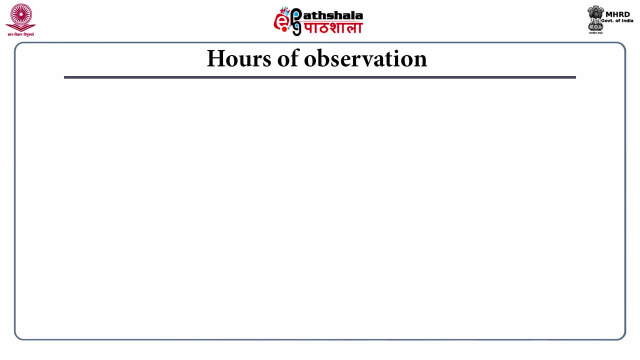 as free air flow. Now, another important thing is hours of observations. In case of surface observatory, regular surface observations are taken at three hourly intervals. The synoptic hours starts at 0 GMT and then observations are taken at every three hour interval. that 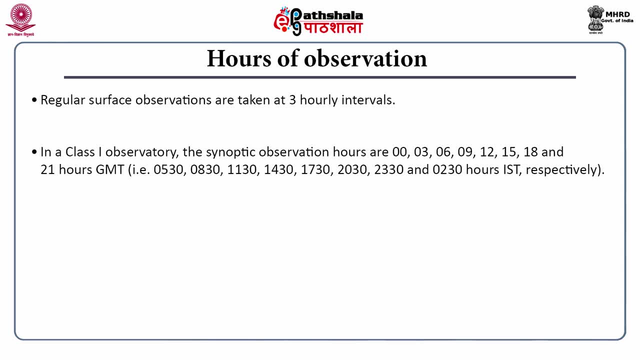 is 6,, 9,, 12, likewise up to 21 GMT. However, in most observatories in India, two observations- one morning observation at 830 hours IST and another afternoon observations at 1730 IST- are recorded For agrometallurgical observatories. morning: 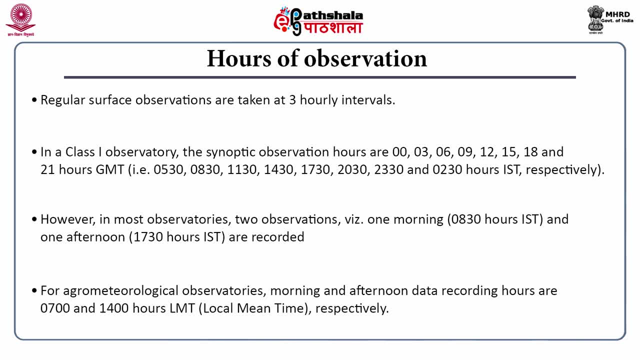 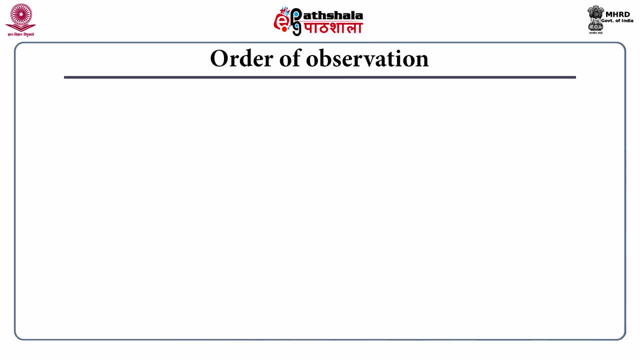 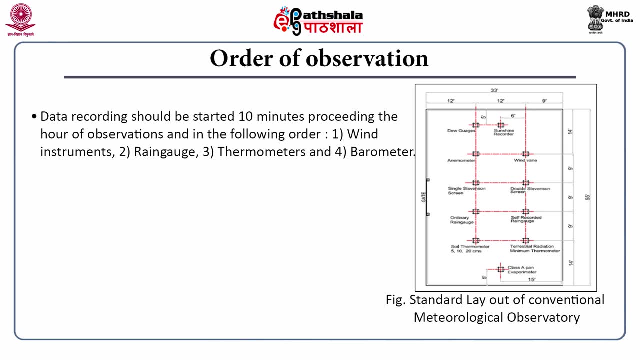 observation is taken at 7 LMT and afternoon observation is taken at 14 LMT. LMT means local mean time. Then in which order the observations should be taken. Data recording should be started 10 minutes preceding the hour of observations and in the following order: first comes 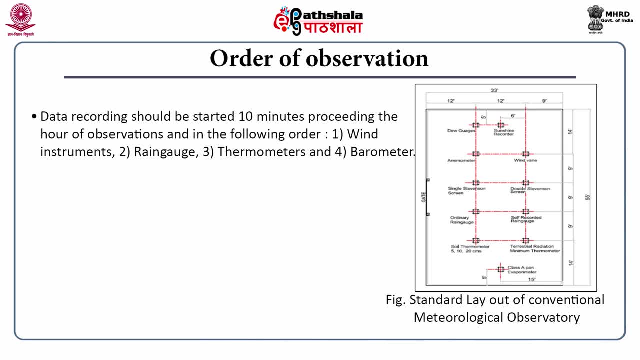 wind instruments, then rain gauge, then thermometers and then barometers. Non-instrumental observations like clouds, visibility, etcetera, should be taken In the interval of three minutes of first and second reading of the anemometer, or else it can be taken before commencing of the instrumental observations. 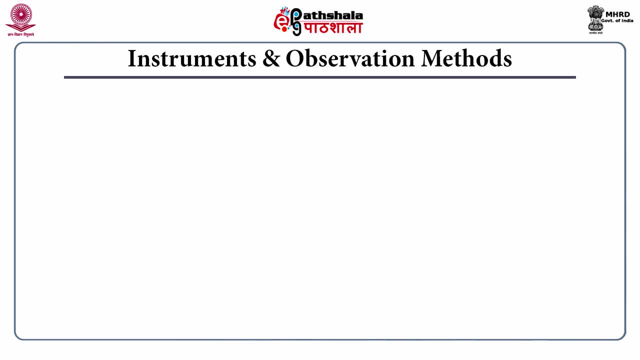 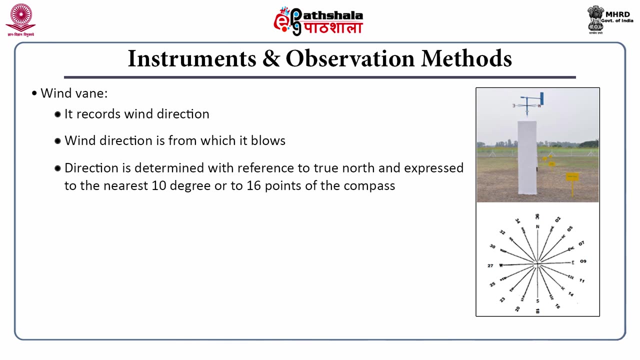 Now the various instruments and the observation methods. Let us discuss with wind vane. Start with wind vane. Wind vane records wind direction. Wind direction is the direction from which wind blows. Direction is determined with reference to true north and expressed to the nearest. 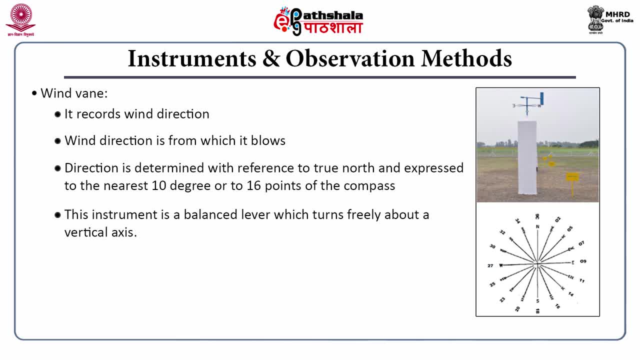 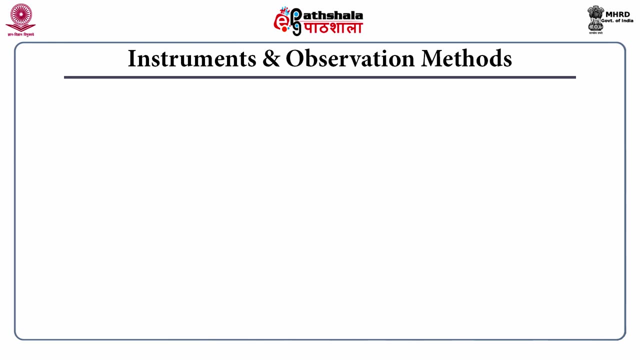 10 degrees or 16 points of the compass. This instrument is a balance-driver which turns freely about a vertical axis Like an arrow. the one end is like an arrow and the other end is like a flat plate, So the narrower end points to the direction from which wind is blowing. Next comes cup anemometer. It. 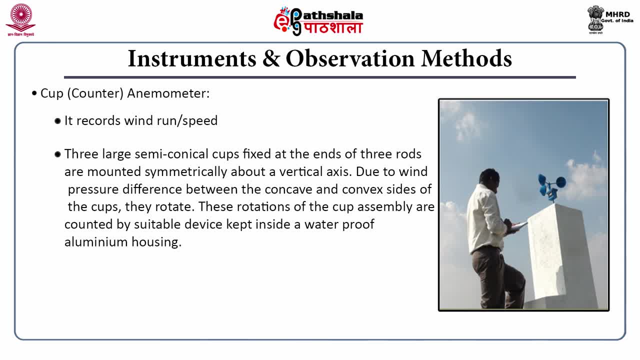 records wind run. There are three large semi-conical cups fixed at the ends of three rods, and these are mounted symmetrically about a vertical axis Due to the wind pressure difference between the concave and concave. the wind pressure difference between the concave and 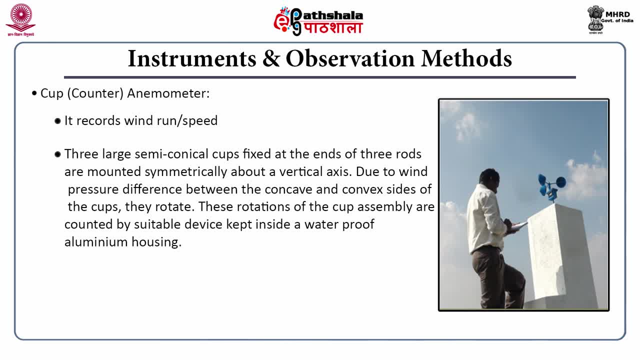 convex sides of the cups, they rotate. These rotations of the cup assembly are counted by suitable device kept inside a waterproof aluminum housing. The counter is read at the beginning and end of a period to obtain the difference. that is, the wind run And then 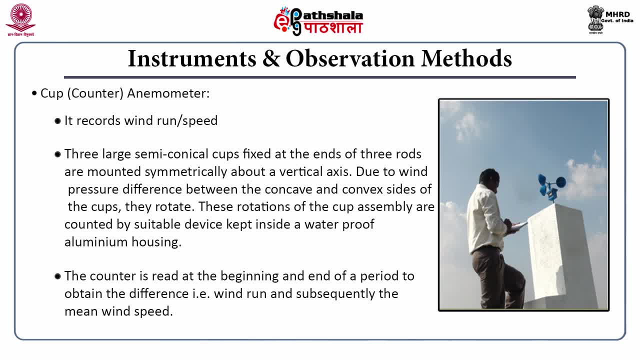 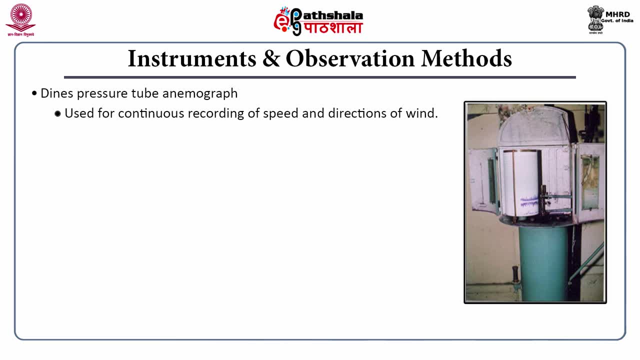 if we divide the wind run by the time period then we can get mean wind speed. Next equipment is dine pressure tube anemograph. It is used for continuous recording of wind speed and directions of wind. The details of wind structure can be known from this kind of equipment, like the occurrence. 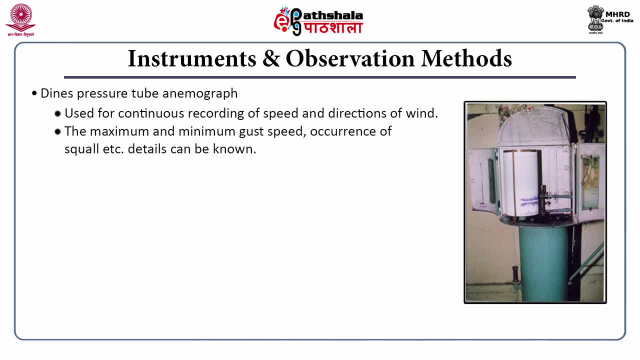 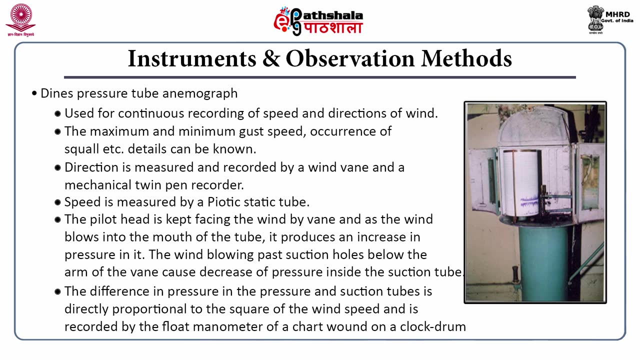 time of occurrence of maximum and minimum gust speed, then occurrence of squall, etc. The direction is measured and recorded by wind vane and a mechanical twin-pane recorder. In case of speed it is measured by piotric static tube. The difference in pressure in the pressure and suction tubes of this equipment. 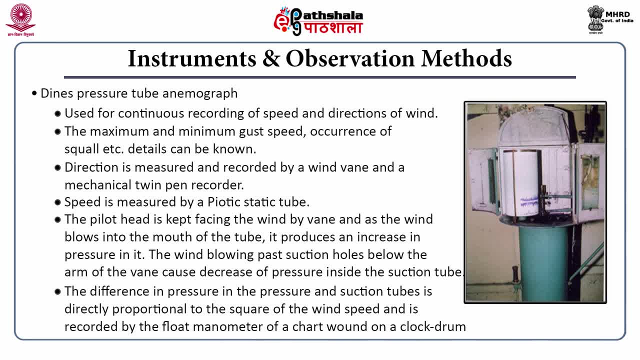 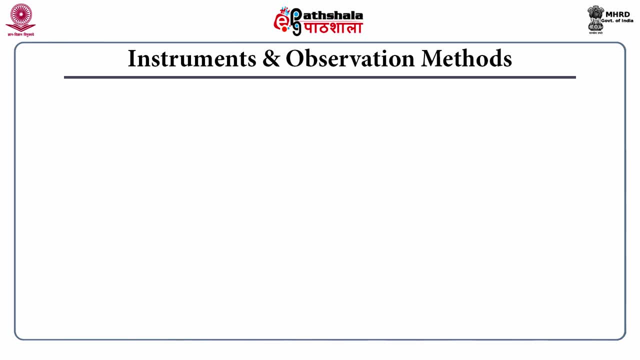 is directly proportional to the square of the wind speed And when the wind speed is is recorded by a float manometer, that is, on a chart which is wound on a clogged drum. The next equipment is ordinary rain gauge. It measures the total amount of rain for a given. 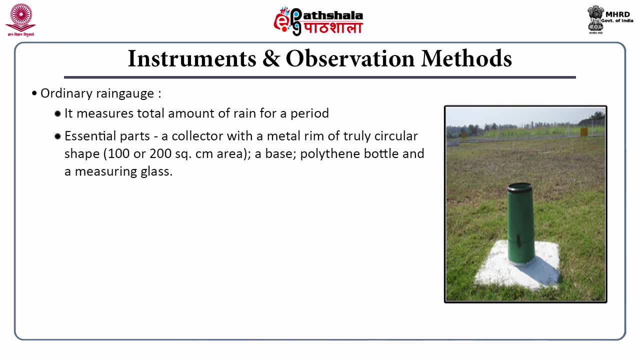 time period. The essential part of it is a collector with a metal rim or of truly circular shape. The size is generally 100 to 200 square centimeter. Then there is a base, a polythene bottle and a measuring glass. The collector and the base are made of FRP, that is, fiber glass. 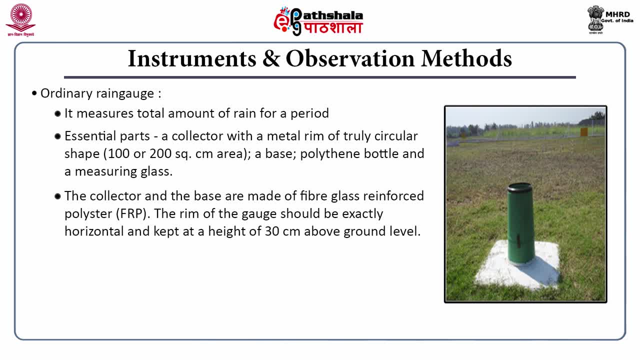 reinforced polyester. The rim of the gauge should be exactly horizontal and kept at a height of 30 centimeter above the ground To measure the rainfall. remove the funnel or collector of the rain gauge, Then take the liquid in a polythene bottle and pour its content in. 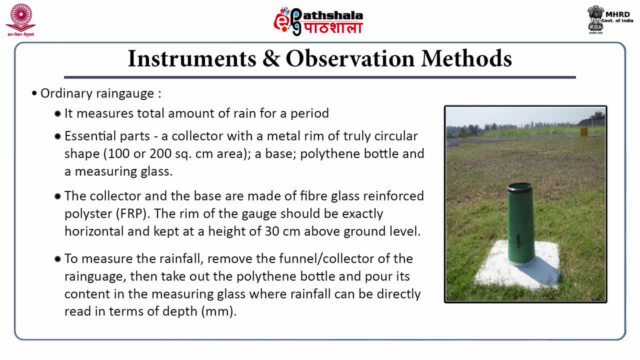 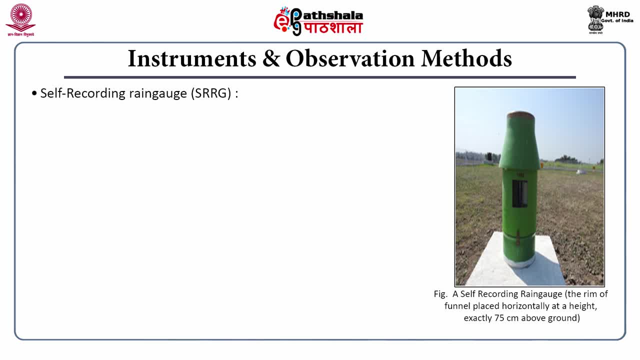 the measuring glass. In the measuring glass it is already graduated and the depth of the rainfall can be directly read. Then comes self-recording rain gauge. It provides continuous recording of the rainfall. The principle governing it is that rainwater entering the gauge. 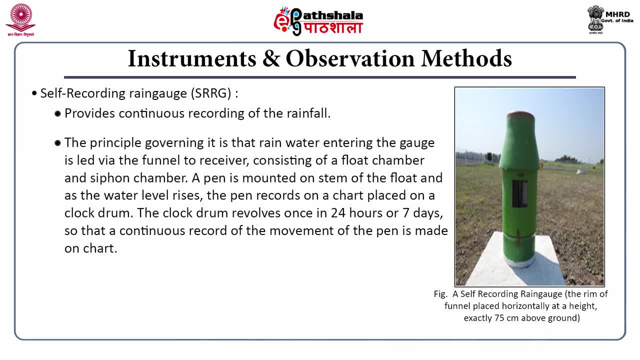 by a funnel to a receiver. The receiver consists of a float chamber and a siphon chamber. A pen is mounted on a stem of the float and, as the water level rises, the pen records on the chart, which is placed on a clogged drum. The clogged drum revolves once in 24 hours or so. 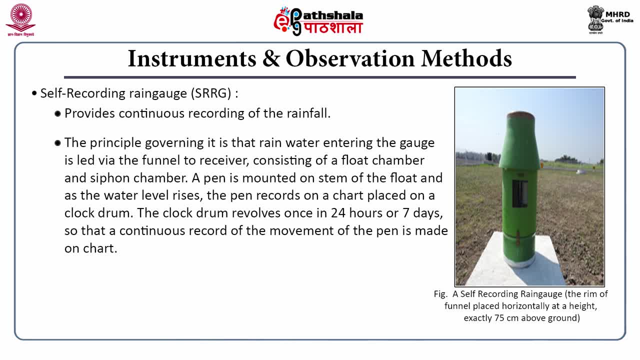 Sometimes it will even fall by several days. Such is how a continuous record of the movement of the pen is made on the chart Once an automatic siphoning occurs, once the pen reaches the top of the chart, and as the rain continues, the pen rises again from the zero line. If there is no. 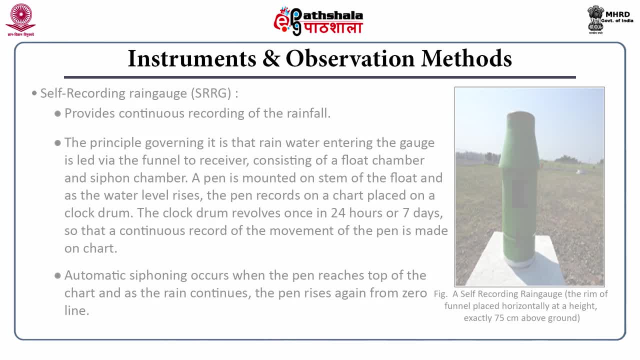 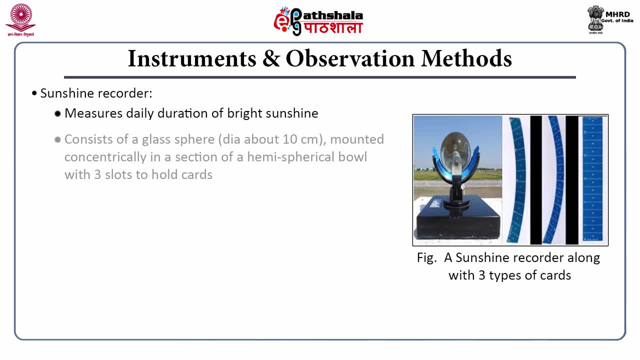 rain. the pen traces the horizontal line. 5. Santiagoectal next equipment is the sunshine recorder. It measures the daily duration of bright sunshine. it consists of a glass sphere which is about 10 centimeter in diameter. this glass sphere is mounted concentrically in a section of a hemispherical bowl which has three slots to 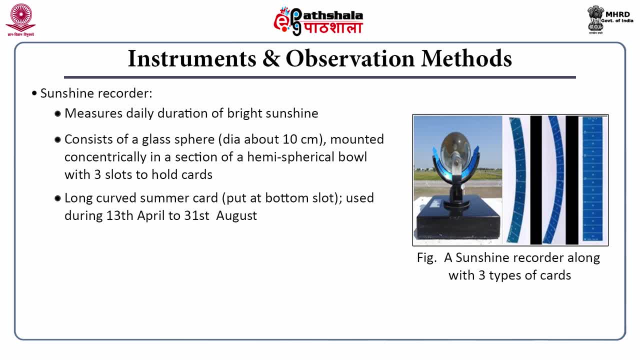 hold three different type of card. during summer time, long curved card is used and this is put at the bottom slot. the time during which it is used is 30th 13th april to 31st august. the next type is card is short curved card. it is used during winter time and it is put at the bottom slot. 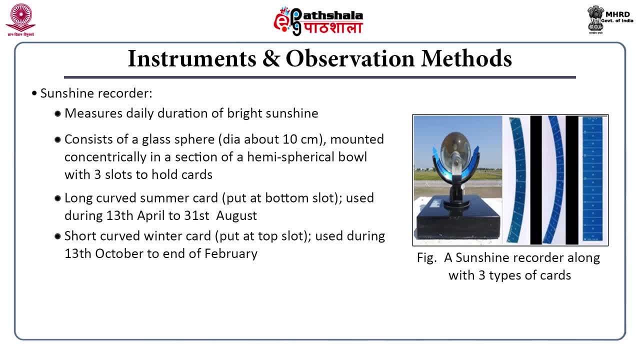 the time during which it is used is 13th october to end of february. the third type is straight or equinoxial card. it is put at the middle slot and used during first march to 12th april and then first september to 12th october. the instrument is kept at open exposed place at three meter height. 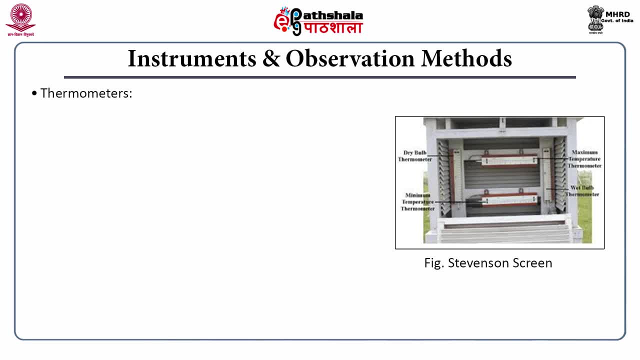 then comes thermometer. there are four type of thermometer: maximum, minimum thermometer and drivable orbital thermometer. these are kept inside a stevenson screen. the stevenson screen is a rectangular box with a sides and door double lowered and the roof is double layered, the base of the 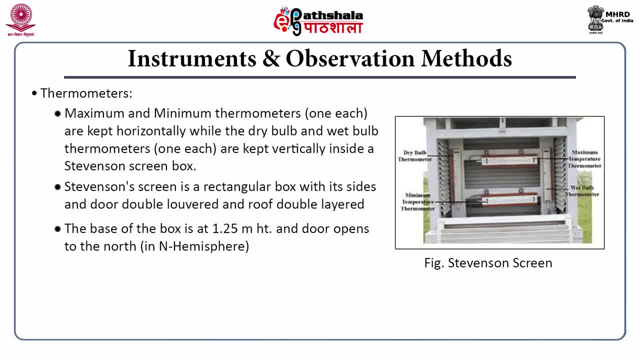 box is at 1.25 meter height and door opens to the north. in the northern hemisphere, such arrangement is to avoid the exposure of direct sun, because the thermometers are meant for not the temperature of direct rays of sun. in all the types of thermometers, mercury. 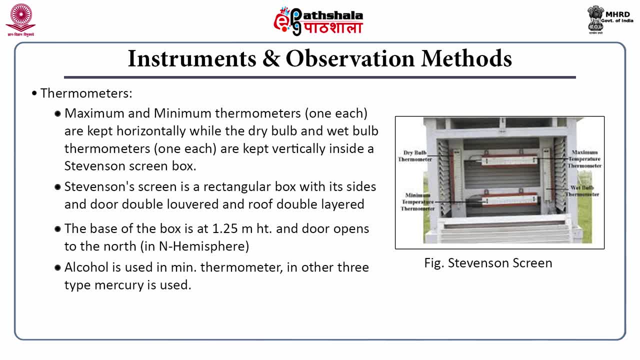 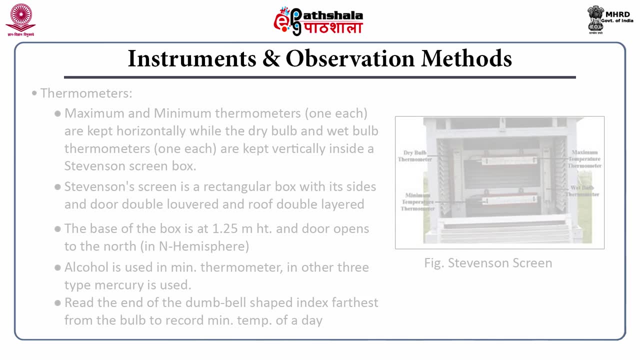 is used as a sensing element, but in case of minimum thermometer alcohol is used. there is a dumbbell separate index inside the your minimum thermometer and we should read the end which is furthest from the bulb, to know the minimum temperature for a given time period. now comes soil thermometers. these are also mercury in glass thermometer which has a bend of. 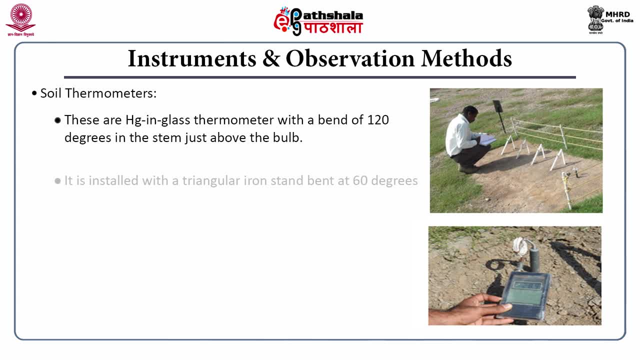 120 degree in the stem, just above the bulb. it is installed with a triangular iron stand bent at 60 degrees. soil thermometers are placed at different depths at surface, then 5 centimeter, 10 centimeter, 20 centimeter and 30 centimeter. these are installed along a line running east to west. 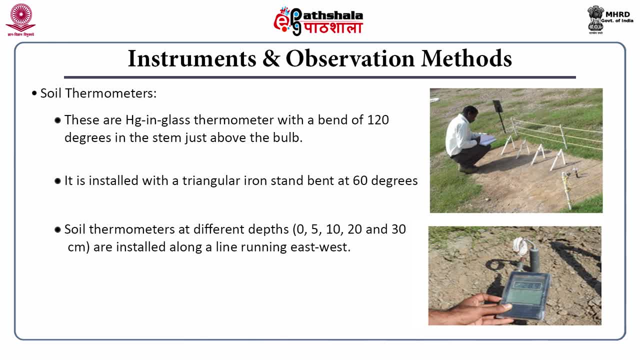 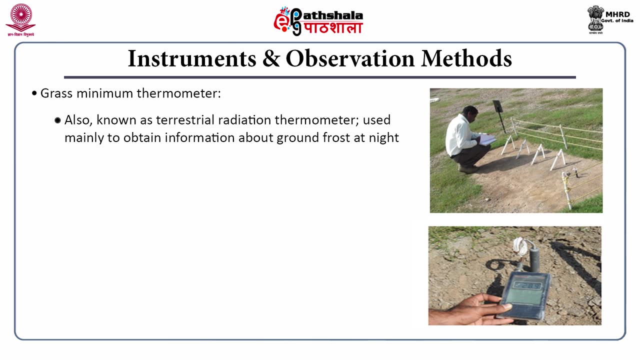 and the measurement is meant up to 30 centimeter, because variations can be seen beyond that depth. the variations are generally less and generally not measured. soil temperature probes with digital meters are also nowadays used to record soil temperature. next is grass minimum thermometer. it is also known as terrestrial radiation thermometer. 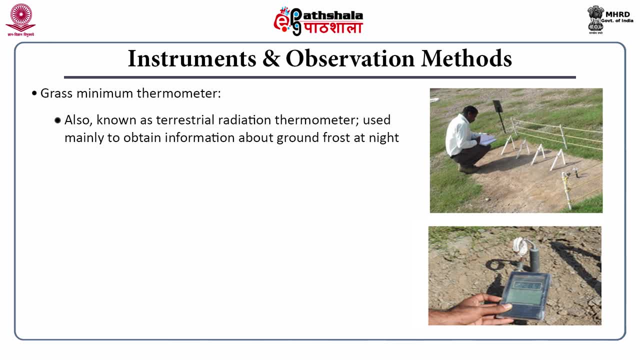 it is used to obtain information about the occurrence of ground frost at night. the instrument is exposed on a plot covered with a short grass 2.5 to 5 centimeter height. it is kept on two y-shaped wooden supports, with the bulb just touching the tips of the. 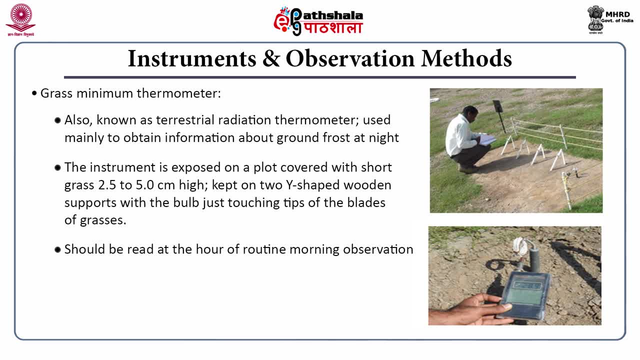 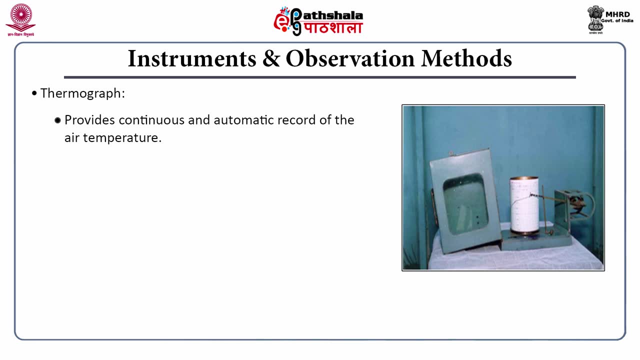 blade of the grass. it should be read at the hour of routine morning observation. after the reading is over, the thermometer is kept inside the screen with bulb downwards until the evening. during evening time it is set again and put over. the grass thermograph provides continuous and automatic record of air temperature. it is placed inside the double estimation screen. 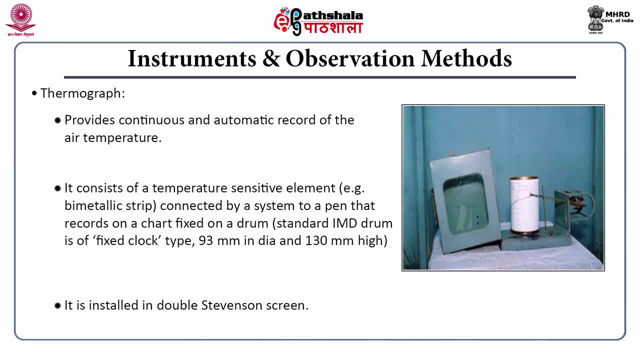 thermograph has a temperature sensing a sensitive element. generally a bi-metallic strip is used as a and it is connected by a system to a pen. That pen records on a chart which is fixed on a drum. The standard IMD drum is a fixed clock type. They have diameter of 93 millimeter. 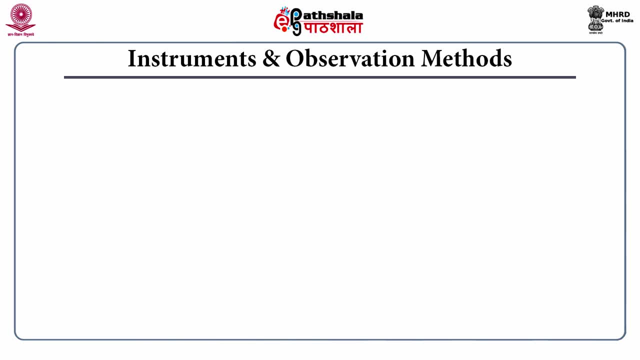 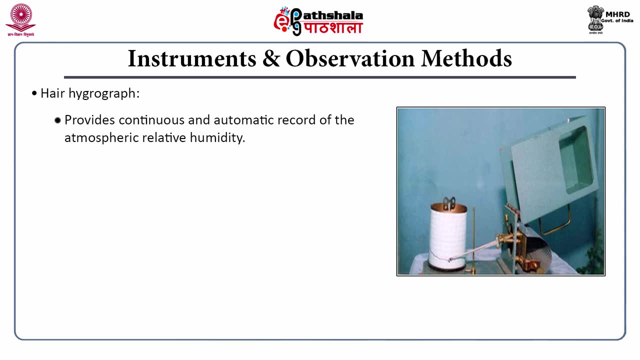 and 130 millimeter in height. The next equipment is hair hygrograph. In case of hair hygrograph, hair is used as a sensing element because human hair is sensitive to relative humidity of the air. Its length changes proportional to the logarithm of the changes in the relative 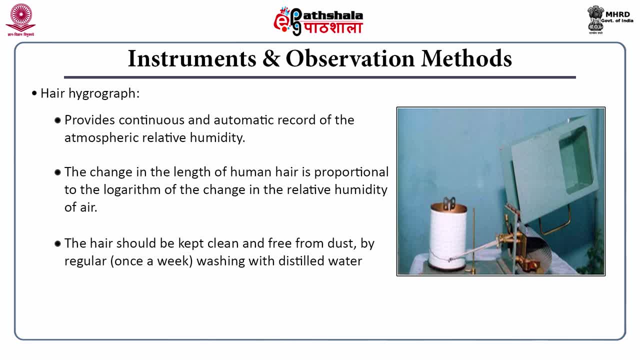 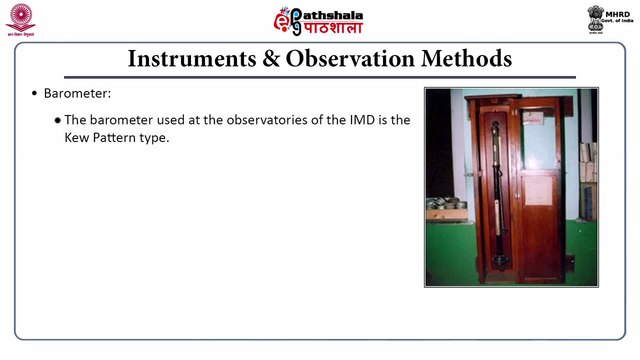 humidity. The hair should be kept clean and free from dust. It should be regularly washed with distilled water. This equipment is also placed inside the double Stevenson screen. Our next equipment is barometer. Barometer is used to measure air pressure. There are 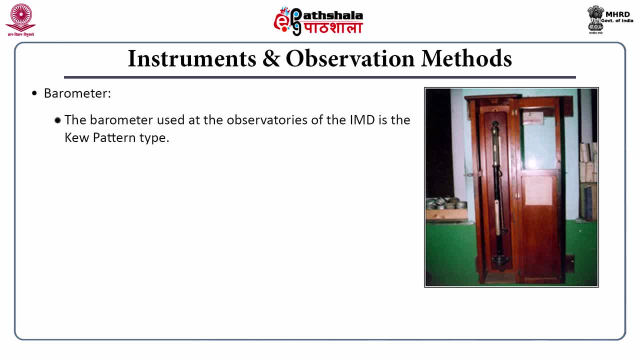 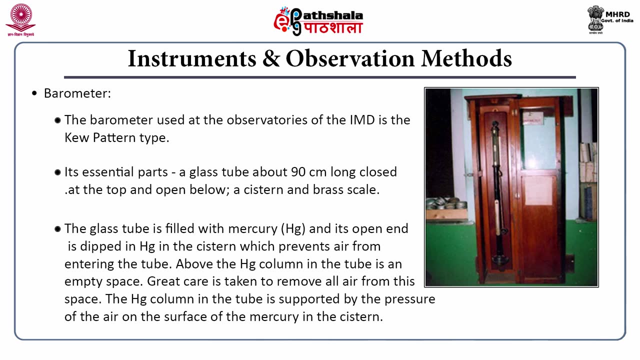 different types, But in most of the IMD observatories cube pattern type barometer is used. Its essential part is a glass tube about 90 centimeter long. The tube is closed at top end and its open is below. Then there is a cistern and a brush scale. The glass tube is filled with mercury. 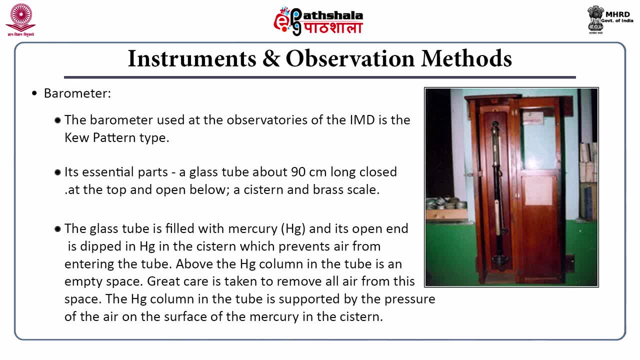 and its open end is dipped in the mercury in the cistern, which prevents air from entering the tube. Above the mercury column in the tube there is an empty space and care should be taken to remove all the air from this space. The mercury column in the tube is supported by the pressure of the air on the surface. 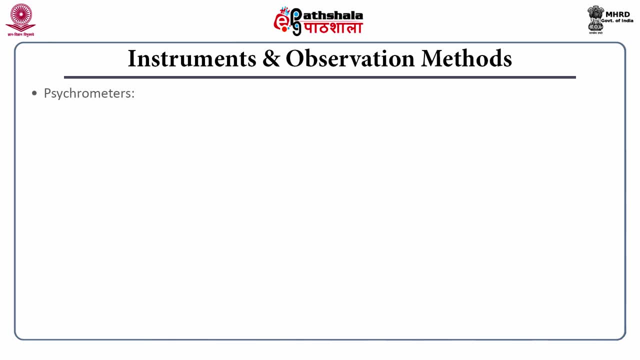 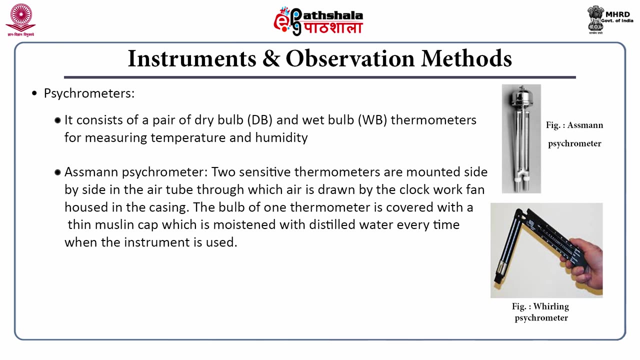 of the mercury in the cistern. Next equipment is psychrometers- Psychrometer generally. it is a pair of dry valve and wet valve thermometers. It is used for measuring temperature and humidity. There are two main types. One is Osmond psychrometer, another is Whirling type psychrometer In case of 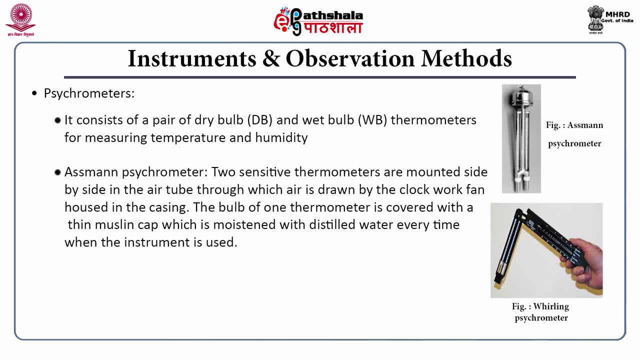 Osmond psychrometer. this dry valve and wet valve is there and air is sucked. This is the air flow, It is the pressure of the air And the pressure of the air is the pressure of the air. This pressure is the pressure of the air And the pressure of the air is the 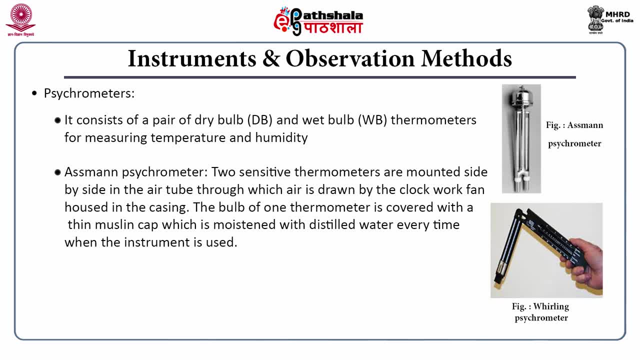 fan. The valve of one thermometer is covered with a thin muslin cap, and each time the cyclometer is used, it should be wetted with distilled water. In case of whirling cyclometer, aspiration is provided by whirling or rotating the thermometers. Desired speed is 5 meter per second, which 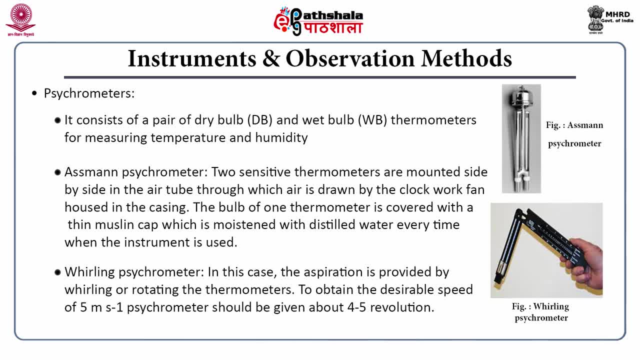 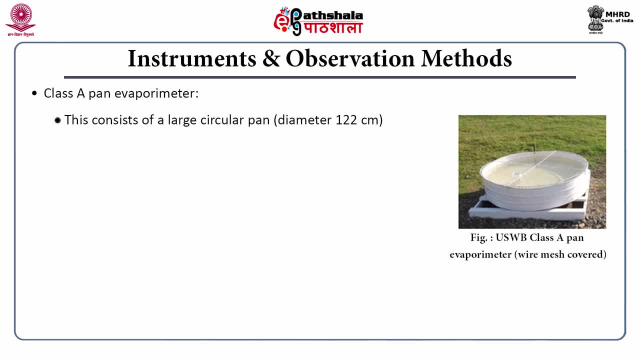 can be obtained by giving 4 to 5 revolutions to this cyclometer. Next equipment is class A pan evaporometer. This consist of a large circular pan with a diameter of 120 centimeter. A filling unit is provided which has three small holes at. 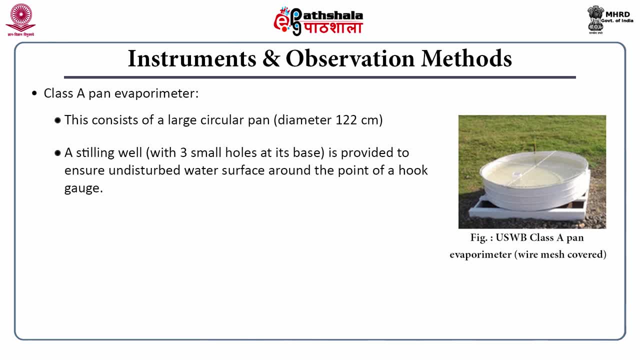 its base, The filling Berkeley is provided to ensure that there is no ripple on its surface, so that the level of water can be accurately read. The amount of water lost by evaporation from the pan during any interval of time is measured by adding known quantities of water. 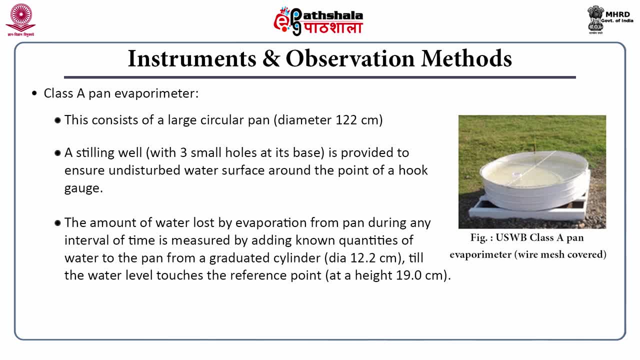 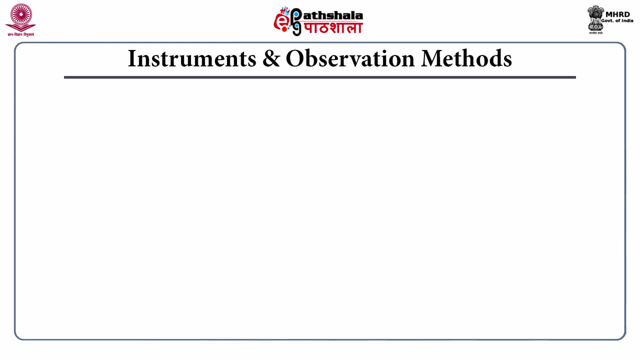 to these pan ó, the pan from a graduated cylinder whose diameter is one-tenth that of the diameter of the open pan. The readings are taken generally at 830 hours IST and in some observatory a second observation at 1430 hours is also taken. Now, how to record evaporation data with a. 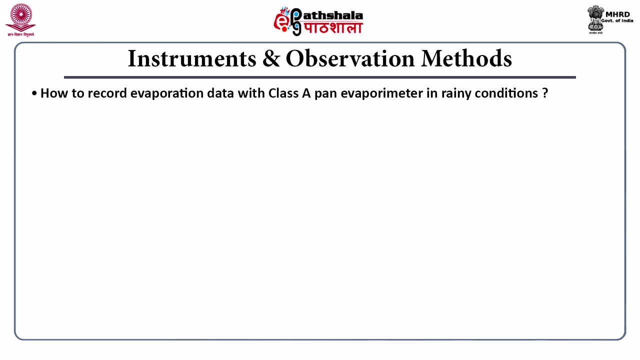 class A pan evapotermeter when there is a rainy condition. Now, there could be light rainy days. there could be heavy rainy days. During light rainy days, when water level is still below the tip of the hook gauge or the reading point, this formula is used. It is: 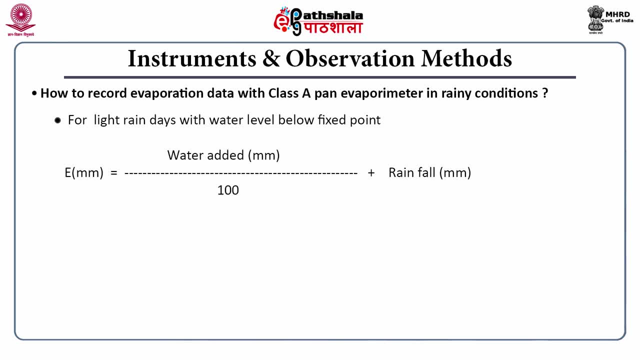 evaporation is equal to water added in millimeter divided by 100, plus rain in millimeter. For heavy rainy days, when we need to remove water to get the water level up to the tip of the hook, we need to use this formula. Evaporation is equal to. 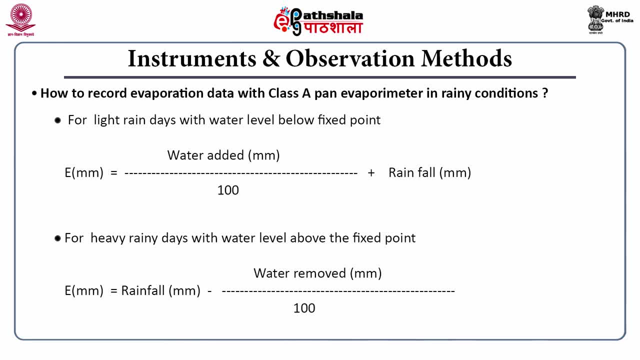 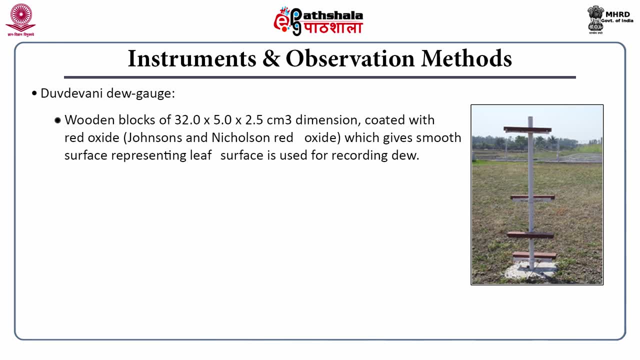 rainfall minus water removed, divided by 100.. Our next equipment is Duke-Dubony dew gauze. It uses wooden blocks of 32 by 5 by 2.5 centimeter cube dimension which is coated with red oxide. The chemical is Johnson's and Nicholson's red oxide. 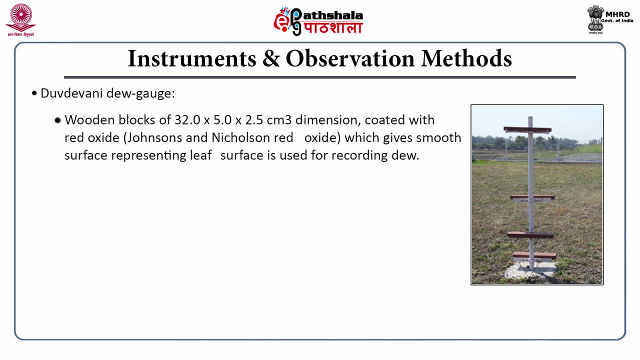 This coating is done to give it a smooth surface so that it can represent the leaf surface. The dew gauges are kept at different heights, namely 5 centimeter, 25 centimeter, 50 centimeter and 100 centimeter above the ground. 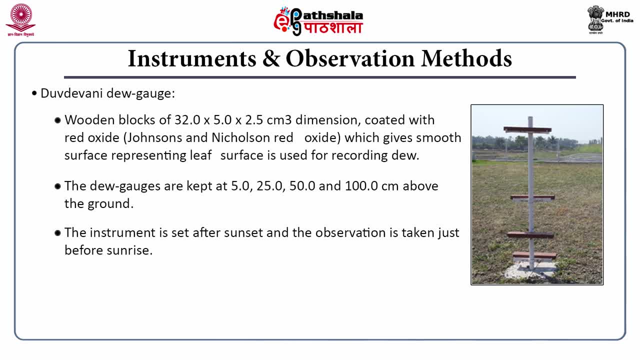 The instrument is set after sunset and the observation is taken just before the sunrise because if you delay then sunrise will cause the evaporation of the dew and we will not get the actual measurement. The amount of dew over the dew gauges are compared to the standard dew photographs which 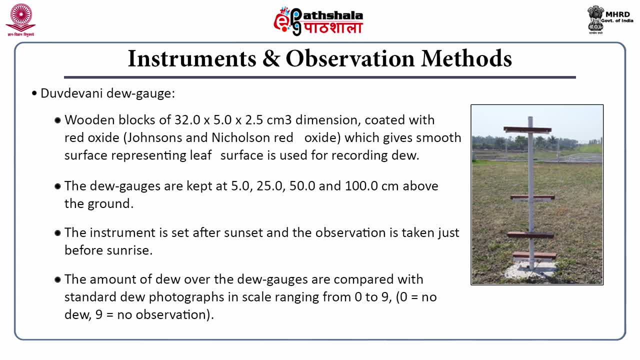 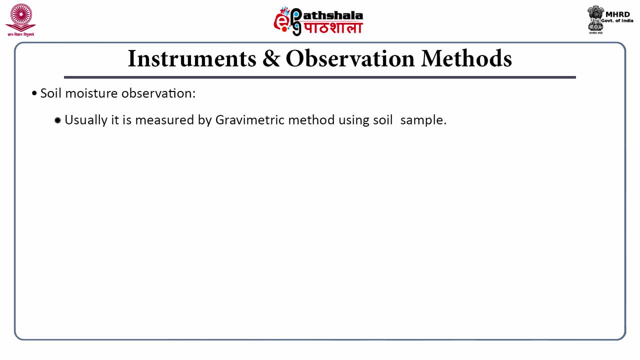 in scale ranging from 1 to 1.5 to 1.5.. From 0 to 9,, 0 means no dew and 9 means no observation. Soil moisture observation is taken in most agglomerate observatories. It is usually measured by gravimetric method. 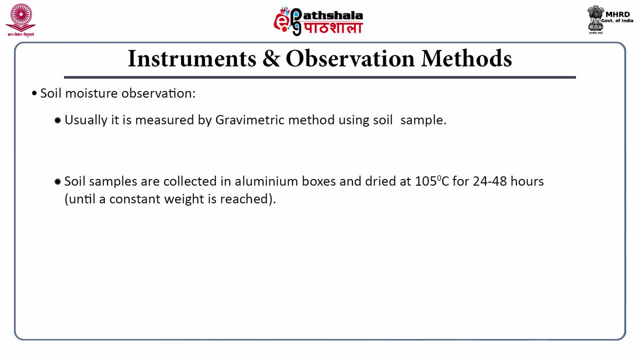 Soil samples are collected in aluminum boxes and those are dried at 105 degree centigrade till a constant weight is reached, Generally based on soil and moisture content. 24 out to 48 hours is required to attain this constant weight, And moisture content is calculated by the weight. 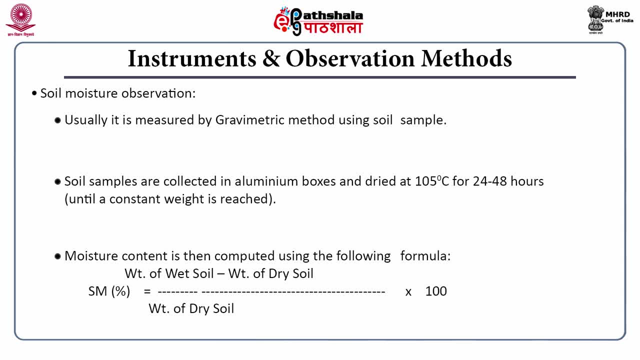 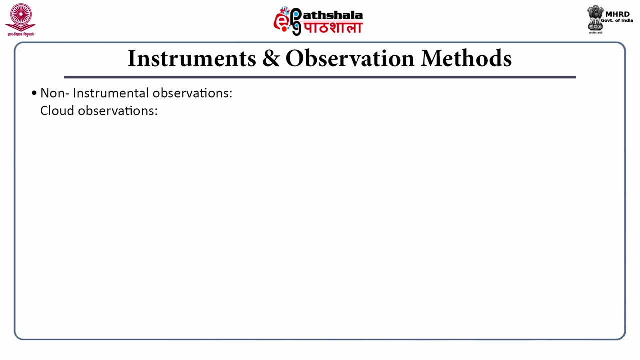 Moisture content is calculated using the following formula: Soil moisture content percentage. gravimetric moisture content is weight of wet soil minus weight of dry soil, divided by wet soil, divided by weight of dry soil into 100.. Now the non-instrumental observations. that means observations which do not require instruments. 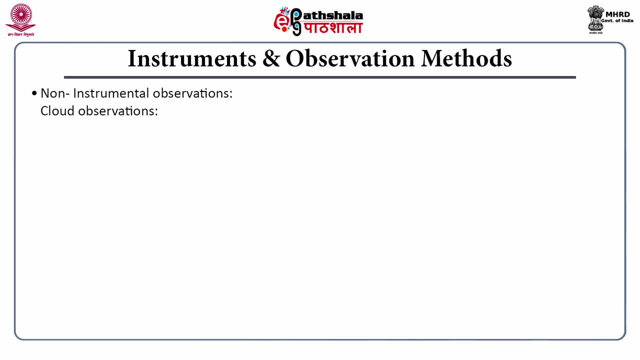 without the aid of the instruments also, these parameters can be measured. One of them is cloud. The cloud amount is reported in terms of octa. It is calculated by the weight of dry soil divided by weight of wet soil, divided by weight of dry soil into 100. 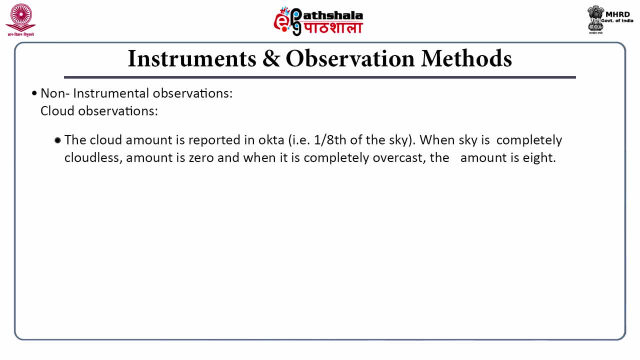 If the sky is completely cloudless, then it is 0 octa. If it is completely overcast, then it is 8 octa. Then main groups of clouds can also be identified, like high cloud, medium cloud or low clouds. Then cloud height, that is the height of the base of the cloud from the ground. 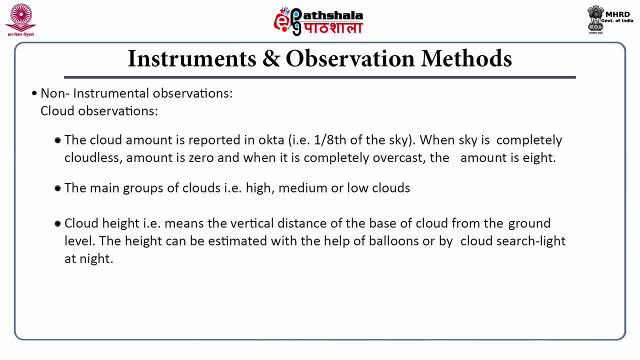 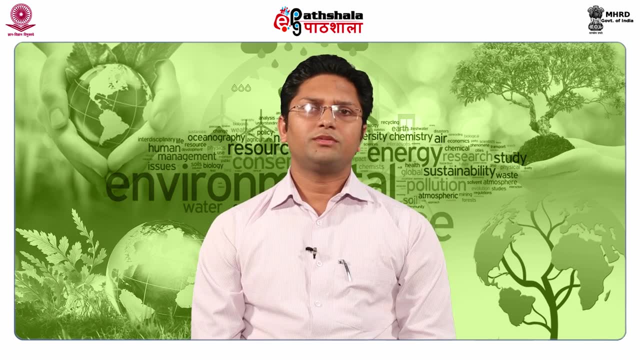 It can be measured, estimated with the help of balloons or, during night time, by search light. also it can be estimated. Direction of movement of cloud is usually can be visually estimated nearest to the 8 point of the compass. To summarize, there are 6 classes of surface meteorological observatories and the data.